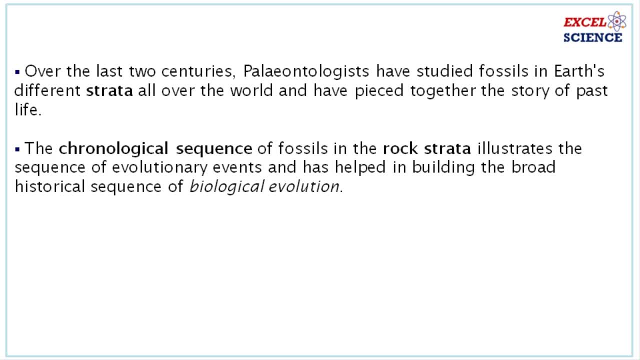 fossils in Earth's different strata All over the world and have pieced together the story of past life. The chronological sequence of fossils in the rocks and scam has been high in modern culture, as well as in history and in the floods of the last century, where Atlantis was known a magical. place to be foundvadge, The chronological sequence of fossils in the rocks, and stating about the Eles you can find in the United States as follows: دم Hi E Clark J Bal cheese. you can TV channel 12. you tai tan應 fellowship處. in the description box below, which has a list. 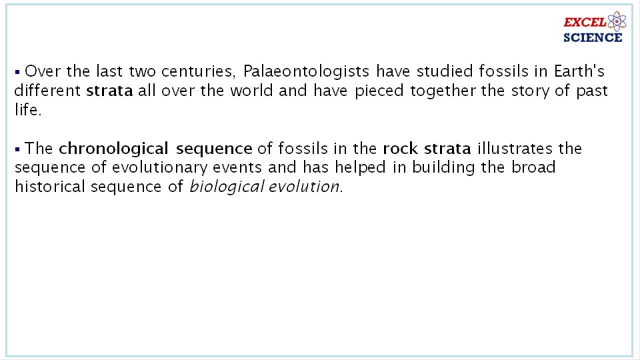 behind the article to subscribe to For more birth information. and don't forget to share with your family hom Cruise to a place- e city verschiedeteam bio- and chat with your friends and friends. strata illustrates the sequence of evolutionary events and has helped in 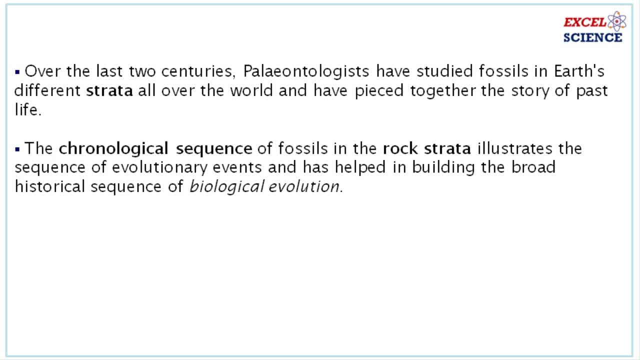 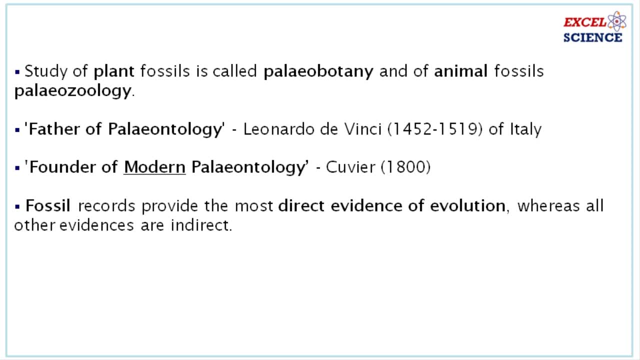 building the broad historical sequence of biological evolution. study of plant fossils is called paleo botany and of animal fossils, paleozoology. Leonardo da Vinci, 1452 to 1519, of Italy, is called the father of paleontology and Cuvier, 1800, is called the founder of the modern paleontology fossil records. 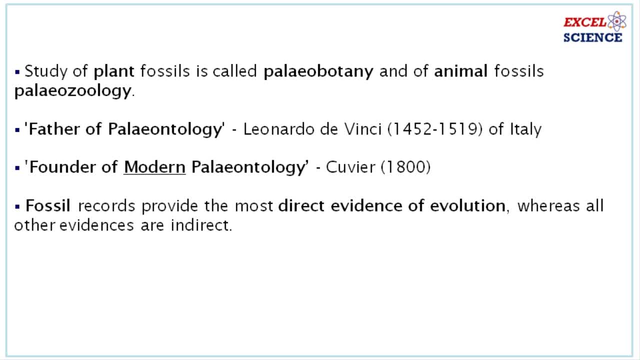 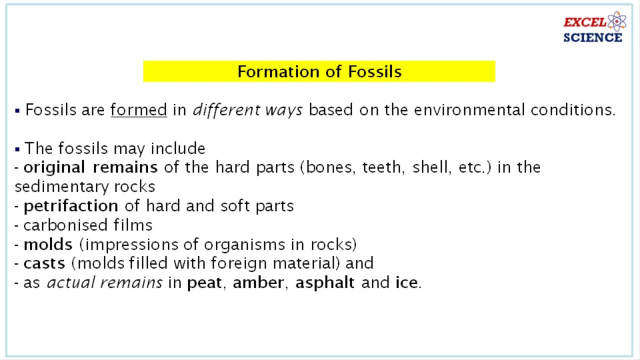 provide the most direct evidence of evolution, whereas all other evidences are indirect formation of fossils. fossils are formed in different ways based on the environmental conditions. the fossils may include original remains of the hard parts, like bones, teeth, shell, etc. in the sedimentary rocks. petrification of hard 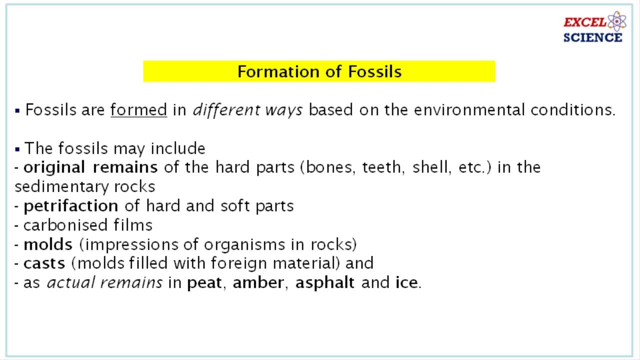 and soft parts, carbonized films, molds, that is, impressions of organisms in rocksis, molds filled with foreign material and actual remains in peat, amber, asphalt and ice. the land animals may also get fossilized in amber that is hard and soft. only partial knowledge is not contained in the whose folks. well, the compound works in the system of paths or the material can as well as be talked about in the science and engineering literature, often in particular research. I'll tell you the different capabilities and capacities of welche, as well as how to and how to get animal fossils. as to the animal and its completeness of animals, ac Prix Logo. 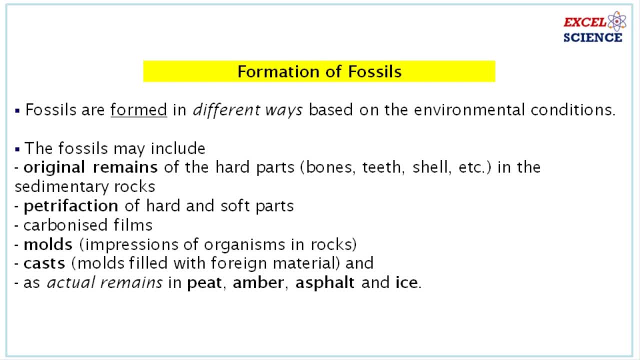 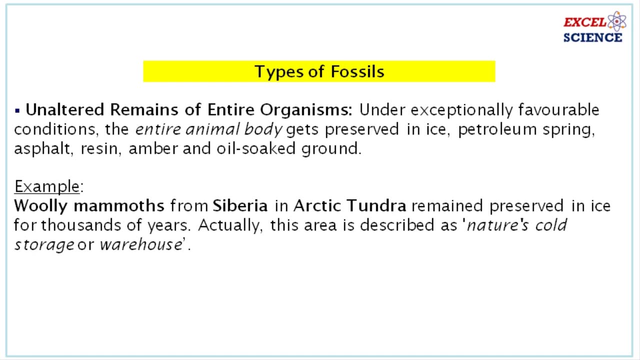 hardened resin, asphalt, hardened tar, volcanic ash, peat, bogs and sand deposits, or in ice. now let's see the types of fossils. fossils are of following types: unaltered remains of entire organisms. petrified fossils, that is, altered fossils, molds and casts, prints or impressions, tracks and frails, coprolites. let's learn about them one by one. first is 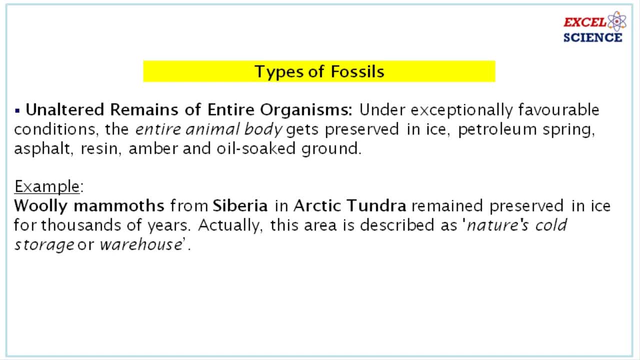 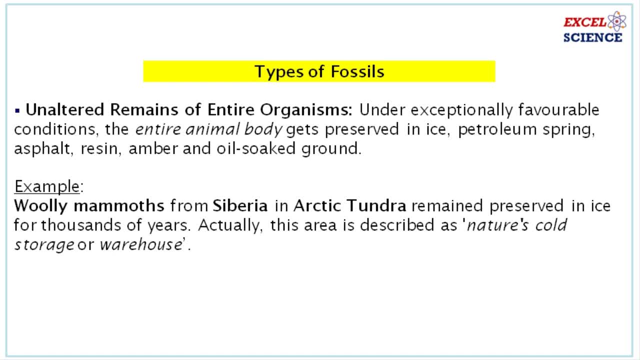 and oil soaked ground woolly mammoths from Siberia in Arctic tundra and oil soaked ground woolly mammoths from Siberia in Arctic tundra remain preserved in ice for thousands. remain preserved in ice for thousands. remain preserved in ice for thousands of years. actually, this area is described as 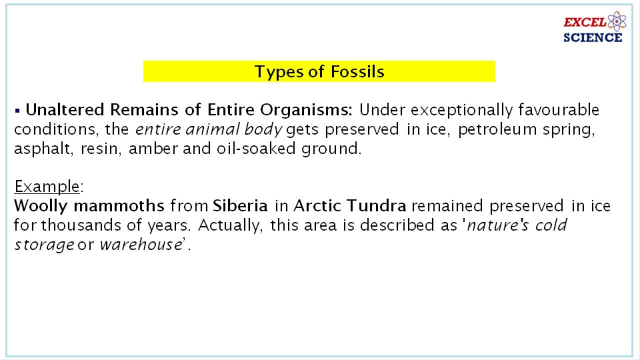 of years. actually, this area is described as of years. actually, this area is described as nature's cold storage or warehouse. next nature's cold storage or warehouse. next nature's cold storage or warehouse. next is petrified fossils that is altered. is petrified fossils: that is altered. 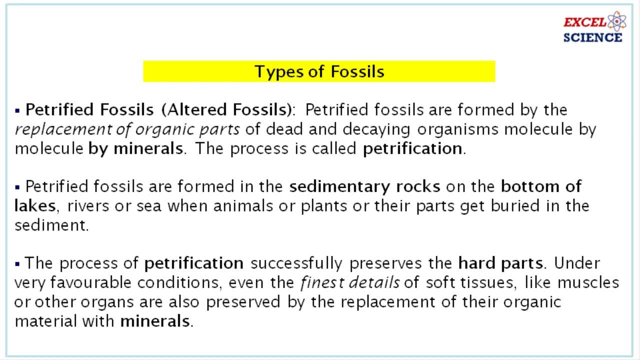 is petrified fossils, that is, altered fossils. petrified fossils are formed by fossils. petrified fossils are formed by fossils. petrified fossils are formed by the replacement of organic parts of dead. the replacement of organic parts of dead. the replacement of organic parts of dead and decaying organisms molecule by. 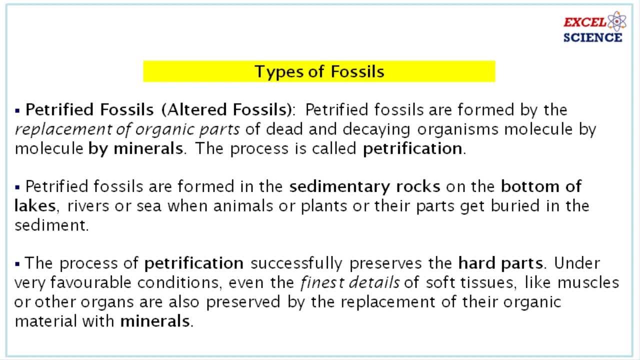 and decaying organisms. molecule by and decaying organisms, molecule by molecule by minerals. molecule by minerals, The process is called petrification. Petrified fossils are formed in the sedimentary rocks on the bottom of lakes, rivers or sea when animals or plants or their parts get buried in the sediment. 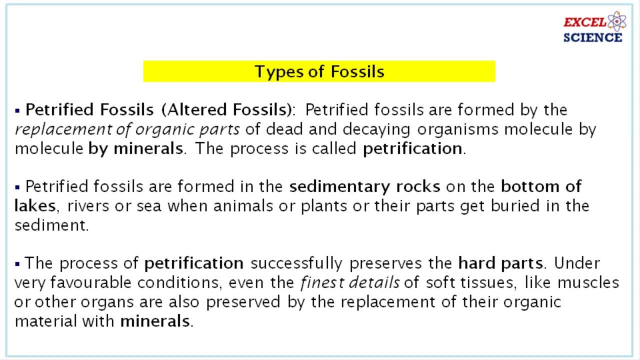 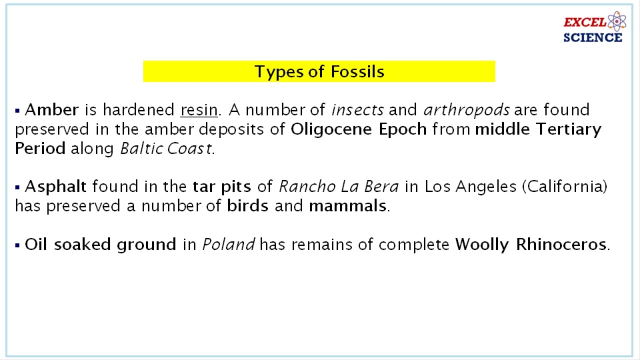 The process of petrification successfully preserves the hard parts Under very favorable conditions. even the finest details or soft tissues like muscles or other organs are also preserved by the replacement of their organic material with minerals. Let's learn about some important points. Amber is hardened resin. A number of insects and orthopods are found preserved in the amber deposits of Oligocene epoch from Middle Tertiary period along Baltic coast. 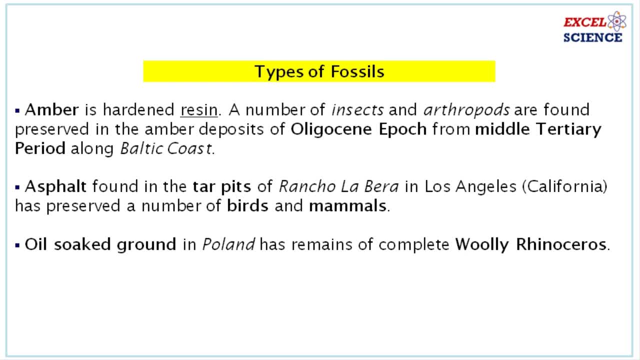 Asphalt. Asphalt is found in the tar pits of Rancho La Vera in Los Angeles, California. It has preserved a number of birds and mammals. Oil-soaked ground- Oil-soaked ground in Poland has remains of complete woolly rhinoceros. 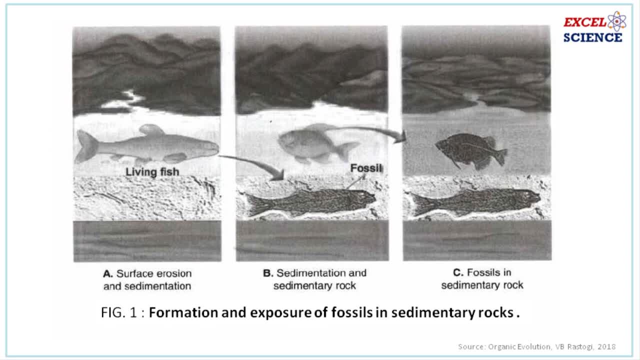 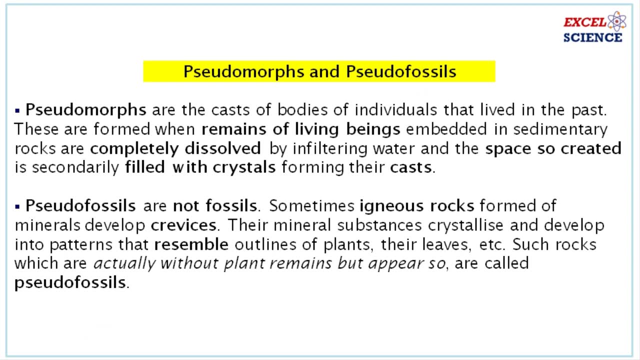 Now let's learn about pseudomorphs and pseudofossils. These are castes of bodies of individuals that lived in the past. These are formed when the remains of living beings embedded in sedimentary rocks are completely dissolved by infiltrating water and the space so created is secondarily filled with crystals forming their castes. 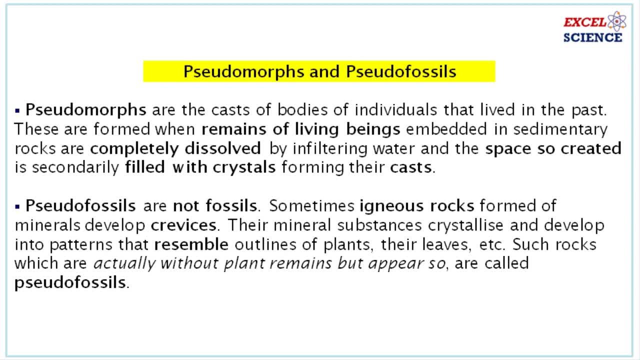 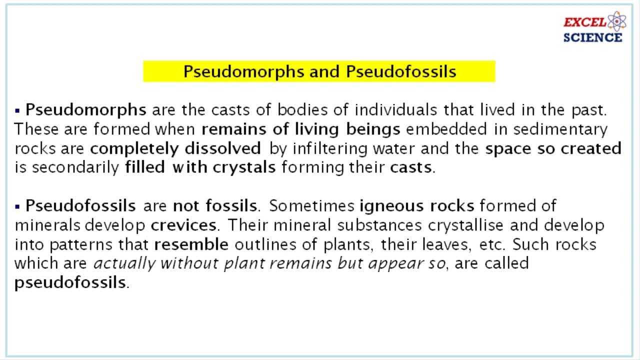 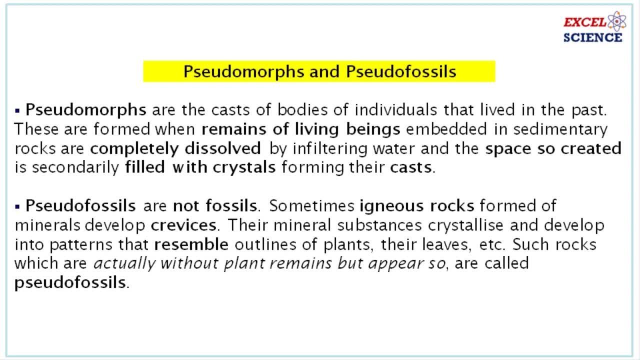 Their mineral substances crystallize and develop into patterns that resemble outlines of plants, their leaves, etc. Their mineral substances crystallize and develop into patterns that resemble outlines of plants, their leaves, etc. that resemble outlines of plants, their leaves, etc.